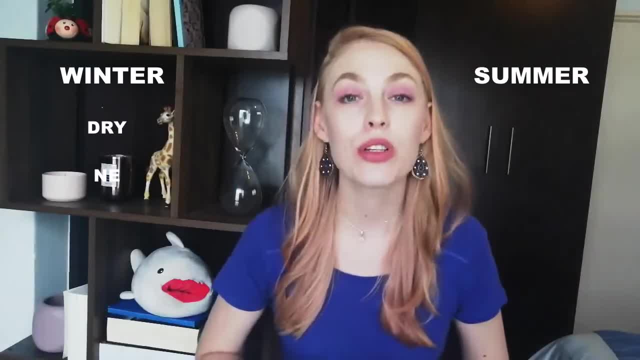 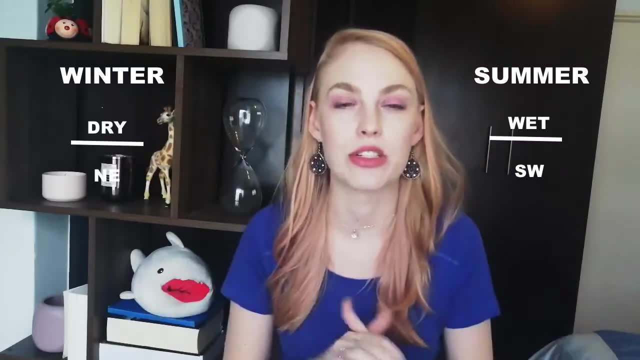 northeast monsoon and our summer monsoon, also known as our southwest or wet monsoon. I'm sure you can already guess what the impact of these two monsoons is going to be. So where does the north, east and southwest come in? In geography, when we are labelling winds, remember a monsoon is a wind. we name it based on where it is coming from. A northeast monsoon means that this wind is coming from the northeast. A southwest monsoon means that this wind is coming from the southwest. And as we look, 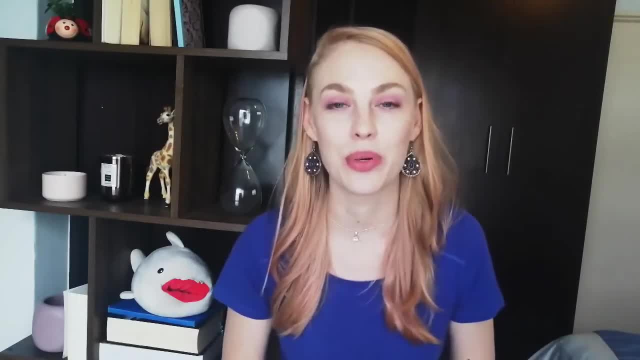 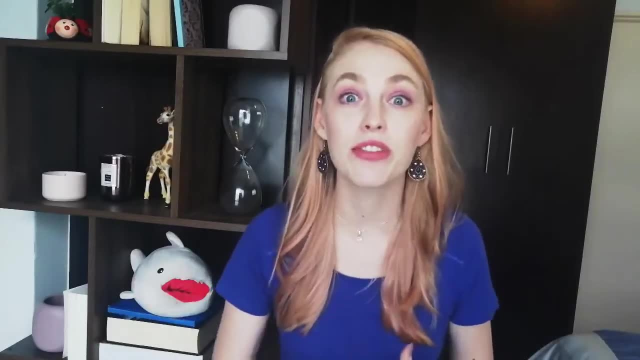 at how these monsoons work, you'll understand what I'm talking about Now. unless you've been living under a rock. you'll know that the northern hemisphere and the southern hemisphere have different seasons at different times of the year. If it is winter in the southern hemisphere. it is summer in the northwest If it is summer in the northern hemisphere, and vice versa. Since we are looking at India, which is in the northern hemisphere, the summer monsoon will happen in the northern hemisphere's summer months. Summer monsoons occur anywhere between June and September. The same thing. goes for the winter monsoon. The winter monsoon will occur anywhere between September and March. Before we can really look at how a summer monsoon and a winter monsoon work. there are four things that we need to understand to help us set this foundation. 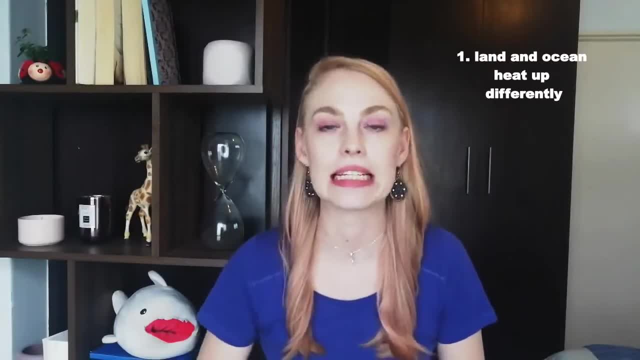 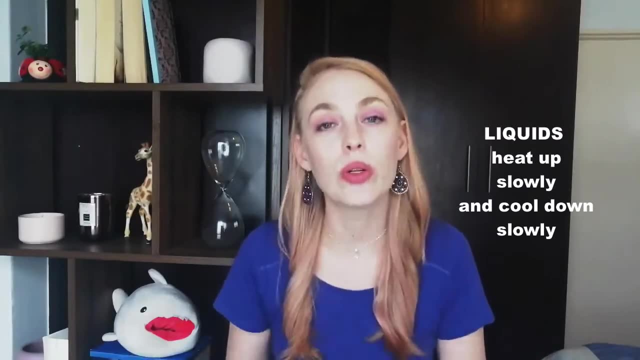 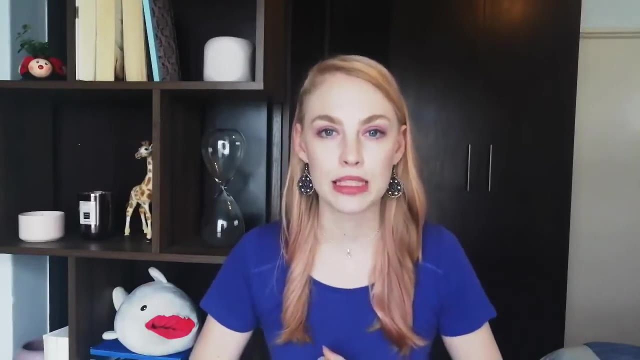 The first thing that we need to know is that the land and the ocean heat up differently. The land is a solid, The ocean is a liquid. Liquids heat up slowly and cool down slowly. Solids heat up quickly and cool down quickly. Let's think about this for a moment On a 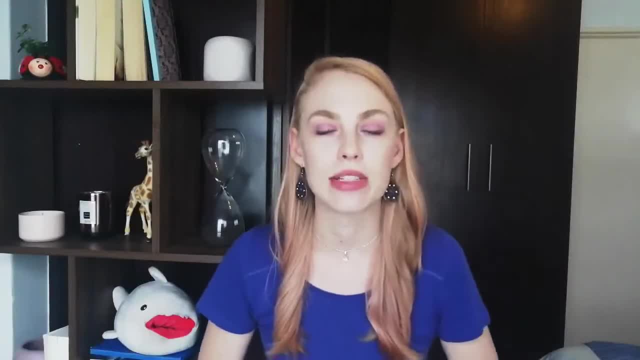 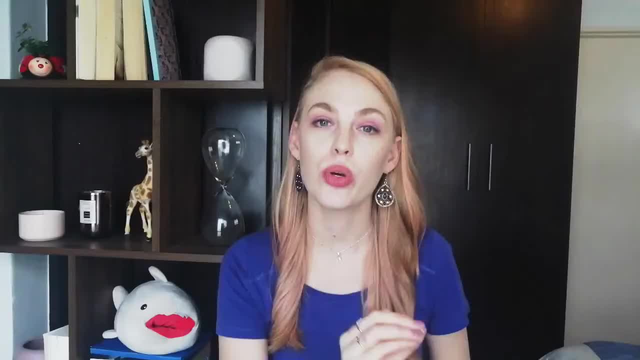 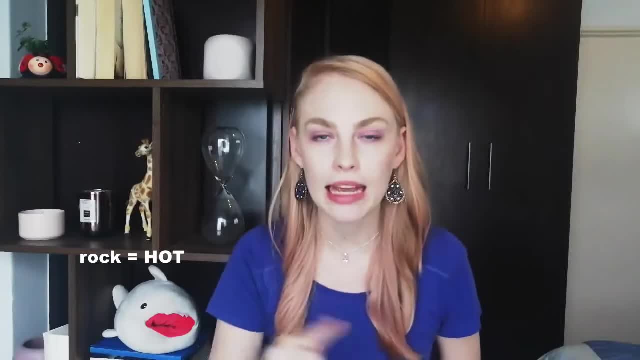 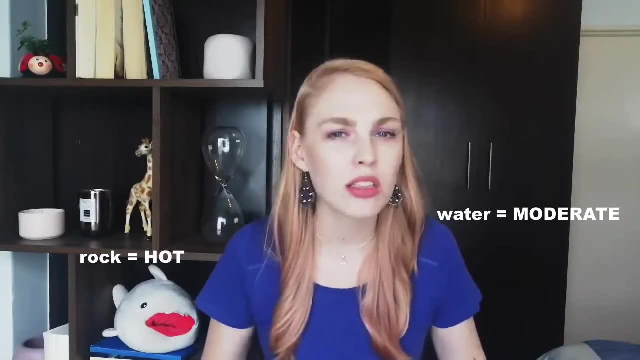 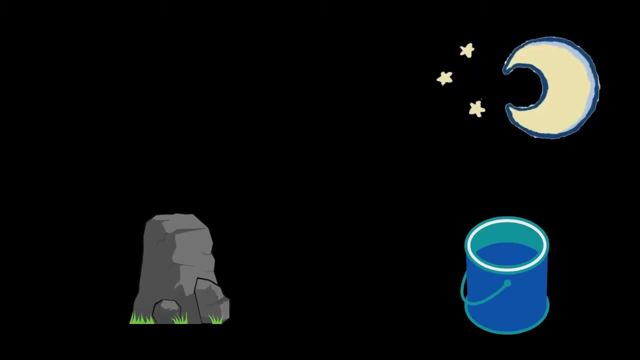 and has absorbed a lot of heat very quickly. If you stick your hand in that bucket of water, it will feel warm, pleasant, Not too hot, not too cold. If you return to that rock and that bucket of water at midnight you will feel that that rock is very cold, It has lost. 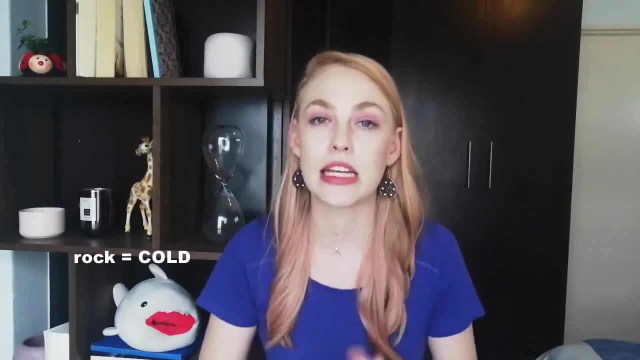 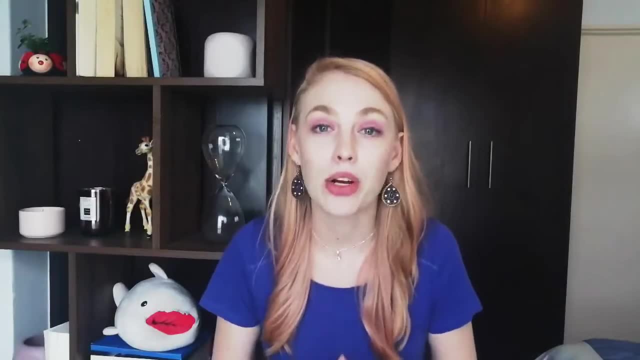 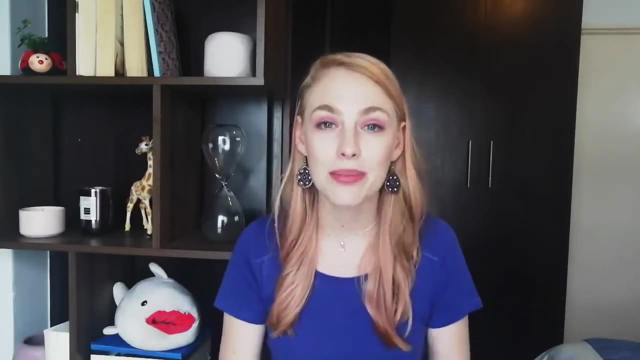 all of that heat very quickly. If you stick your hand in the bucket of water, it will feel around about the same temperature that it did at midday, and that is because liquids retain heat longer. Now the same thing happens on a large scale over our landmass and our ocean. Our land heats up quickly and 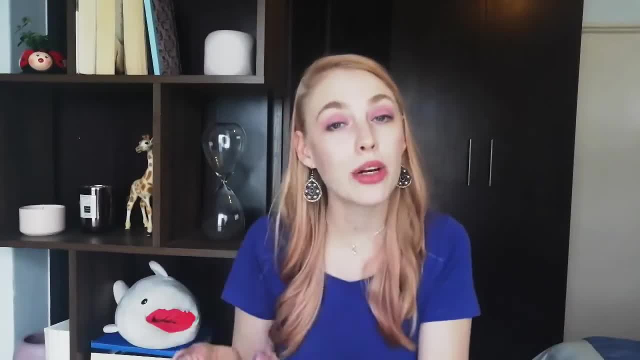 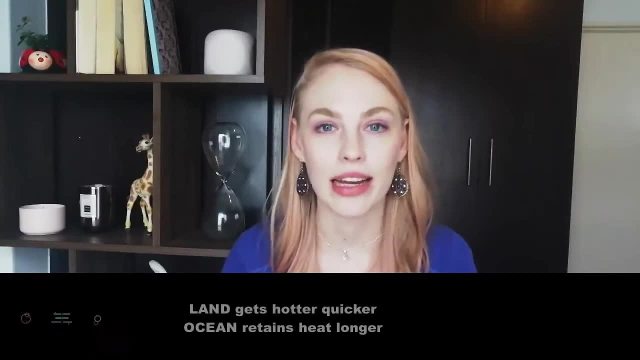 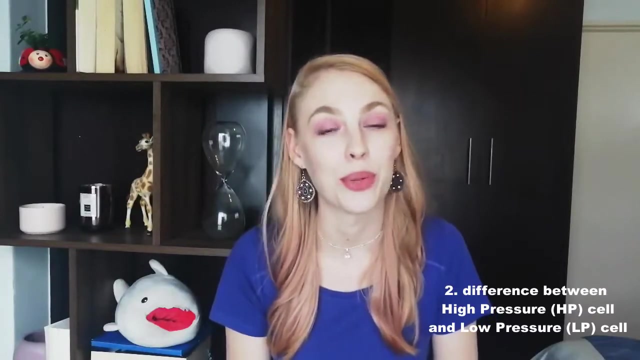 cools down quickly, whereas our ocean warms up slowly and cools down slowly. In other words, the land gets hotter quicker, but the ocean retains heat longer. The second thing that we need to know is the difference between a high-pressure and a low-pressure cell. A high-pressure cell is associated with cold air. Cold air is 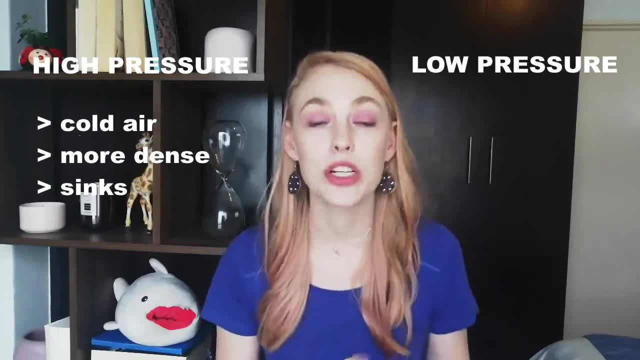 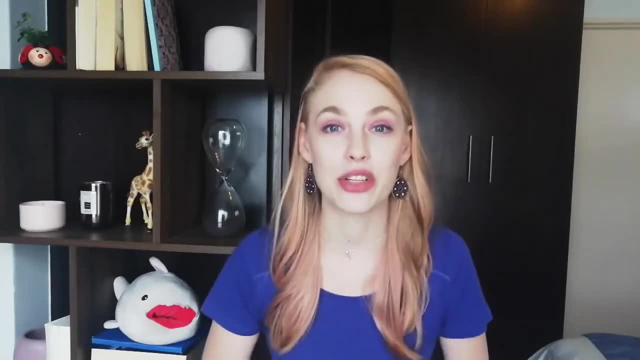 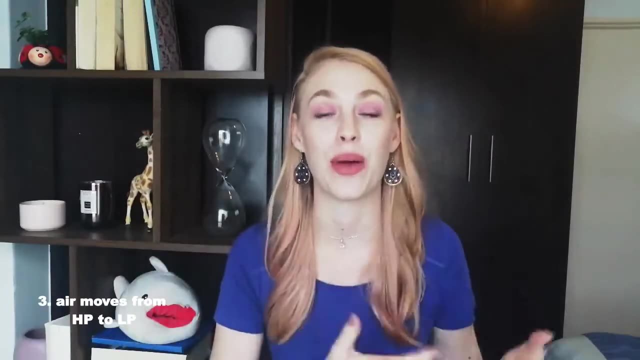 more dense and it sinks. A low-pressure cell is associated with warm air. Warm air is less dense and it rises. The third thing that you need to keep in mind, which is actually our goal and rule for this lesson, is that air always moves from a high pressure to a 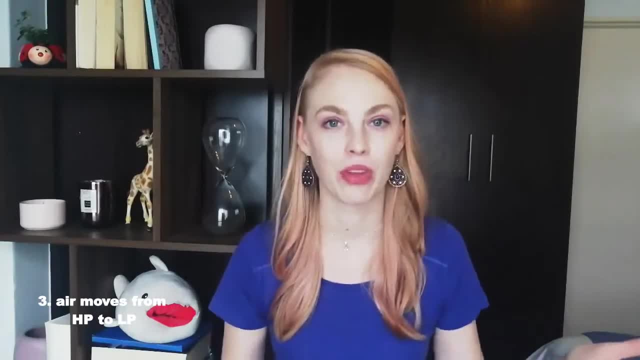 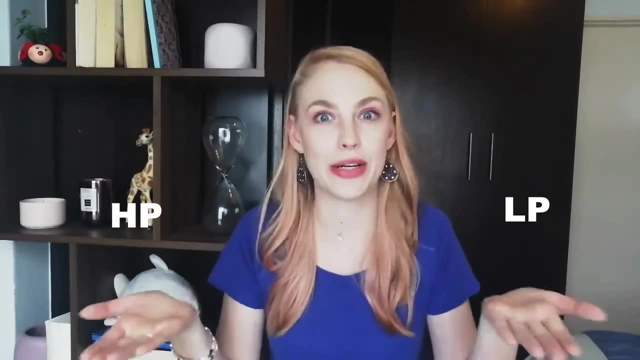 low pressure. Let me explain. Let's pretend, on this side we have a low pressure cell and on this side we have a high-pressure cell. We just learnt that a high-pressure cell is associated with cold air that is sinking. So you need to. 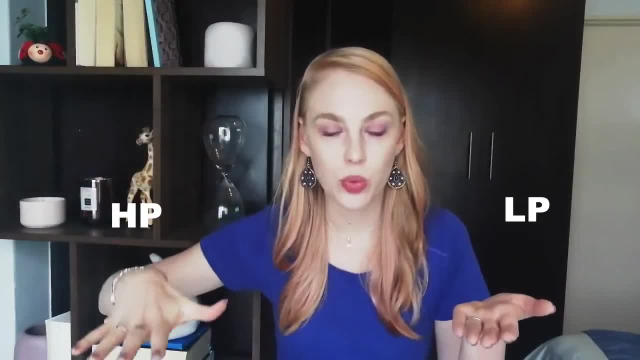 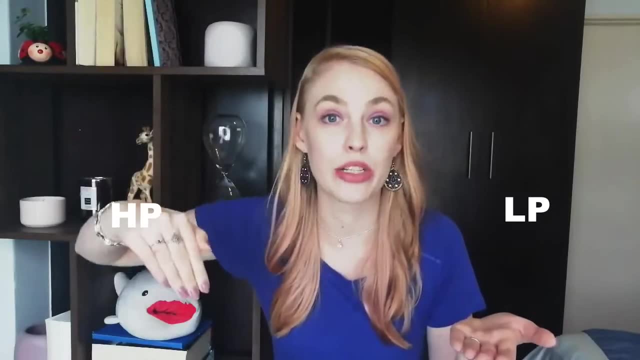 picture this cold air sinking towards the ground. Now, this air can't go past the ground. As soon as it hits the ground, it's going to diverge and move along the Earth's surface. Alright, so this is what we have happening over here. 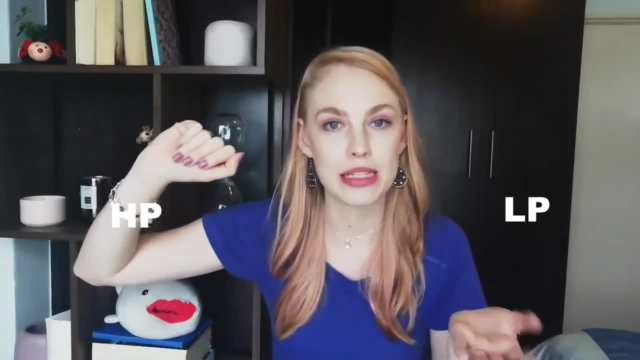 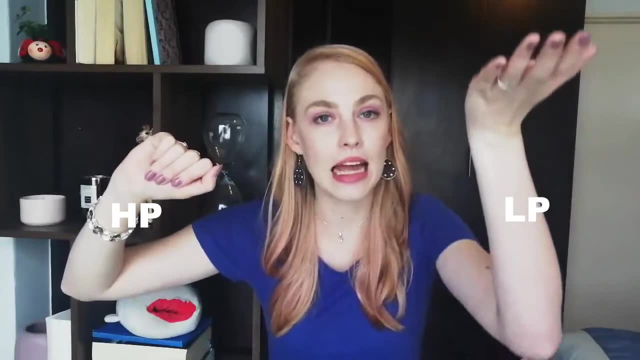 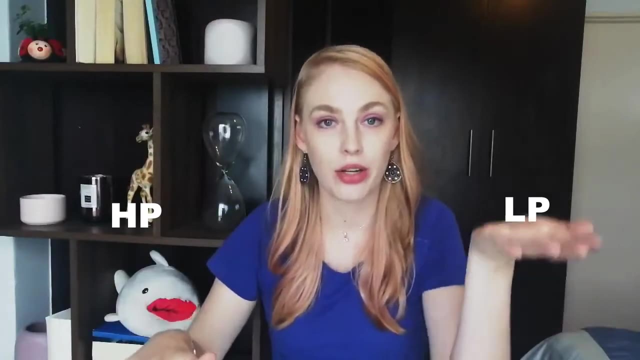 Now let's have a look at our low-pressure cell for a moment. Our low-pressure cell is associated with rising air, So this warm air is going to be rising up. Okay, so we have over here our high-pressure sinking air, Our low-pressure rising air. As soon as 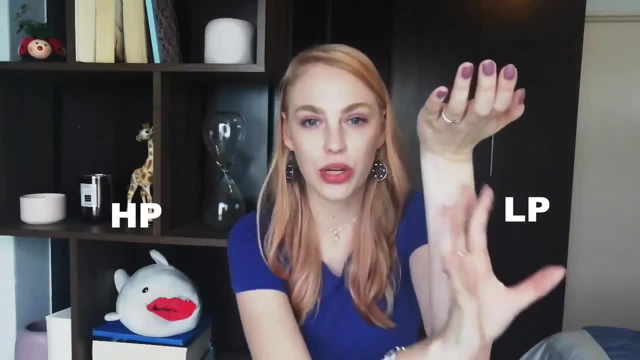 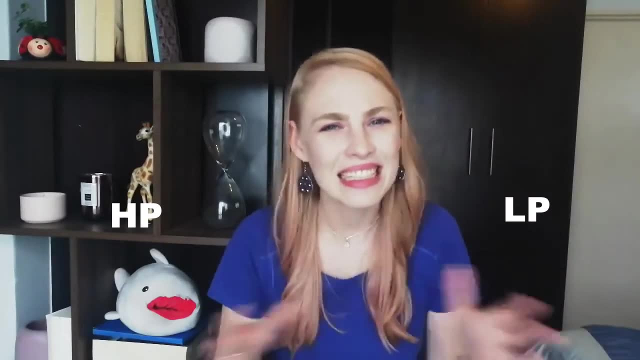 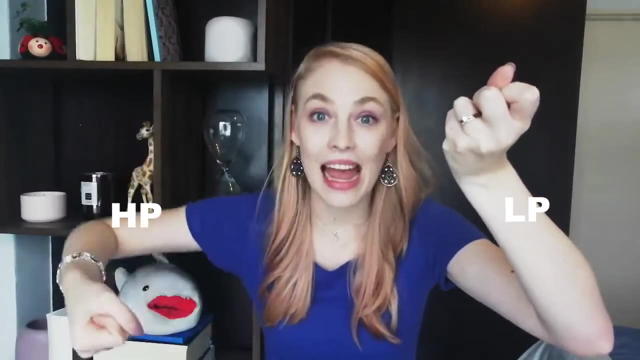 this air rises up, something needs to come and replace it. We can't have a vacuum. A vacuum is a space where no matter exists, and that doesn't happen on Earth. As this air moves up, this cold air that is now sinking and moving along, 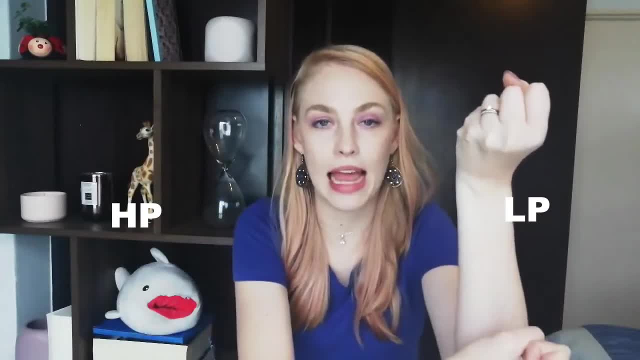 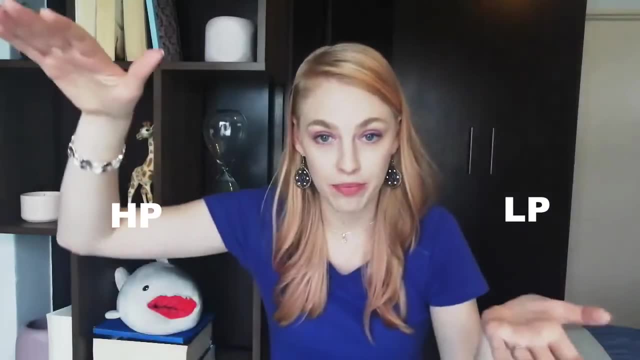 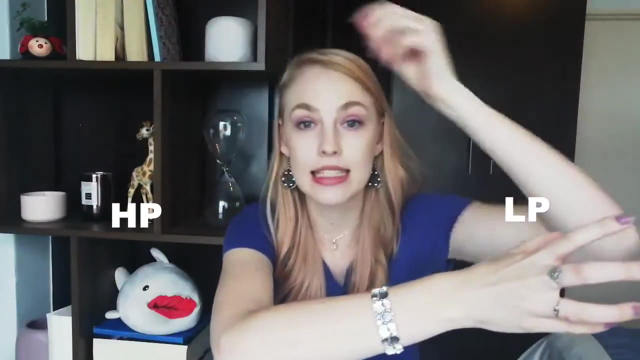 our Earth's surface is going to move towards this empty space and that is why air always moves from a high pressure to a low pressure, So we have a vacuum of this air that is sinking and rising. This air is coming in to replace it and you can see that we have air moving from a high pressure to a low. 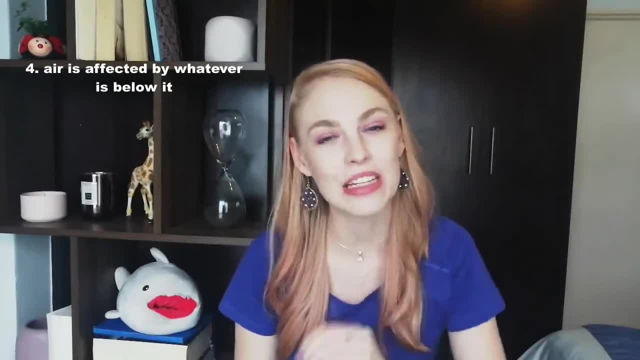 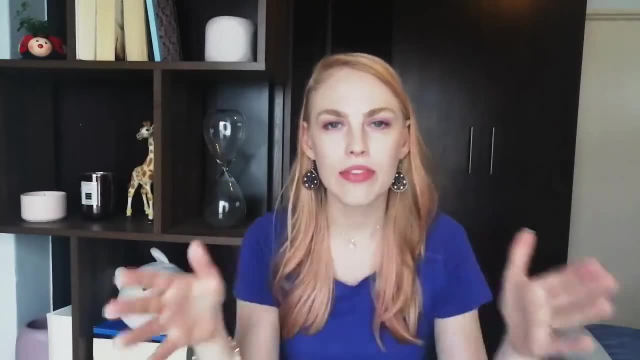 pressure. The fourth thing that you need to know before we can get into monsoons is that air is affected by whatever is below it. You can even do this experiment at home. Fill up your basin with a boiling water. Please do not put your 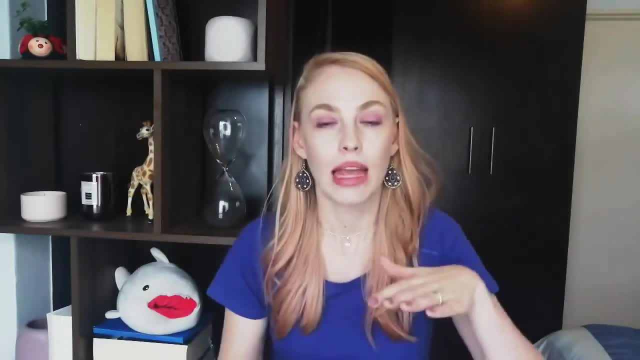 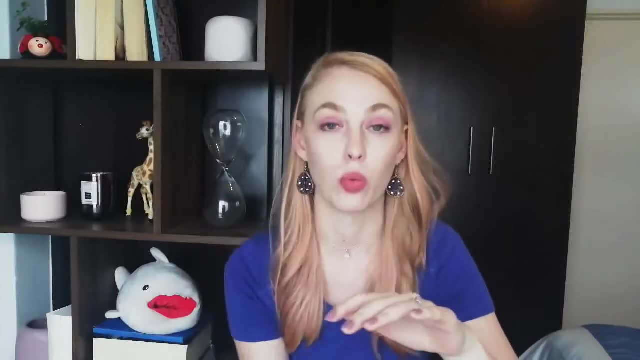 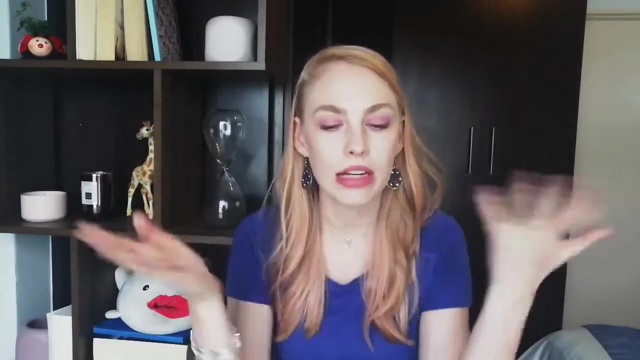 hand in the boiling water. Disclaimer: If you hover your hand above that boiling water, you will feel that the air is warm. So the water is very hot and it has affected the air above it, making the air warm. Now get rid of that hot water. If you fill your basin up with a whole. bunch of ice cubes and you hover your hand above those ice cubes, it will feel cold. The cold ice cubes have affected the air above it, and so the air now feels cold. So we can apply the same principle to monsoons If our land is hot. 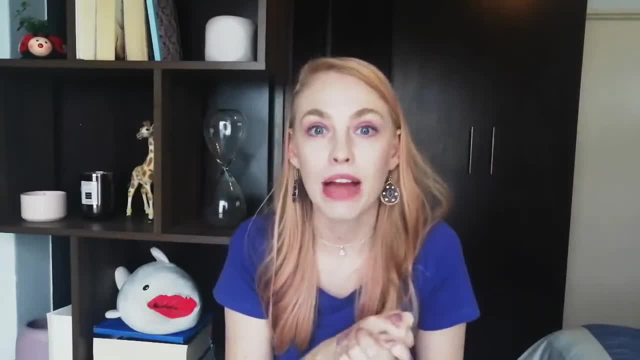 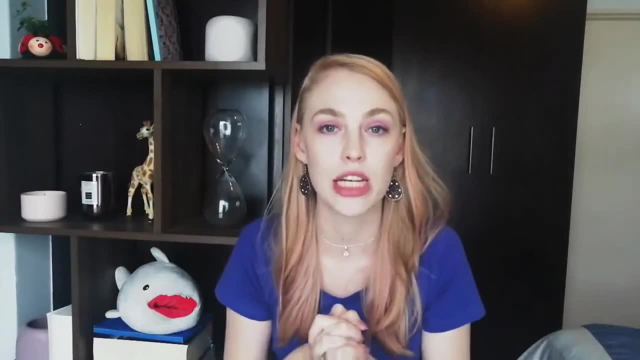 the air above that land is hot. If our ocean is cold, the air above the ocean is cold, Alright, so those are the four things that you need to know before we can jump into monsoons. Now we can look at the difference between a winter. 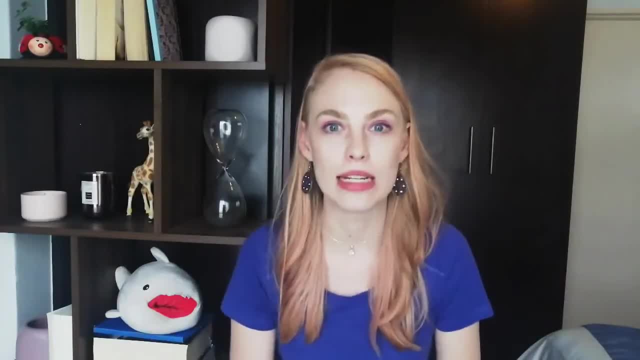 monsoon and a summer monsoon. Let's start off with our winter monsoon. In winter, the landmass doesn't get any colder than the summer monsoon, So we need to know what it really is. The winter monsoon can be as hot, so there is cooler air over the. land. Remember that cold air is associated with a high pressure cell. In comparison to the land, the ocean is much warmer. This means that we have warmer air over the ocean, which is associated with a low pressure cell. Don't forget our golden rule: air always moves from. 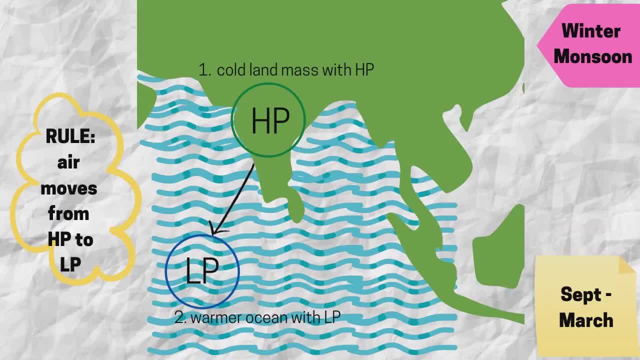 a high pressure to a low pressure. This means that during a winter monsoon, air moves from the land to the sea. So cool air over the land does the job and there is a strong pressure- the ocean. Have a look where this wind is coming from. Our air is coming from the northeast. This makes sense why our winter monsoon is also known as the northeast monsoon. The air that is coming from the land is very cold and dry. Cold, dry air is not associated with cloud formation and it is not associated with rain. This means that winter monsoons result in low rainfall, dry conditions. 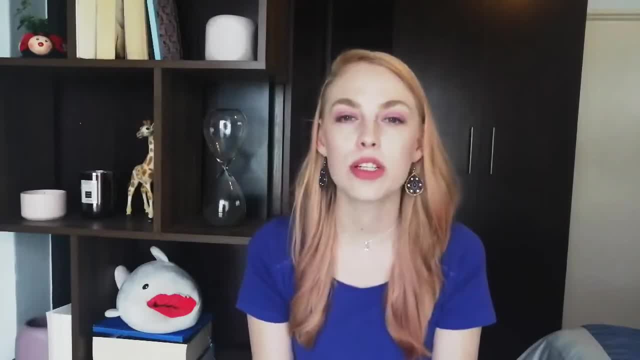 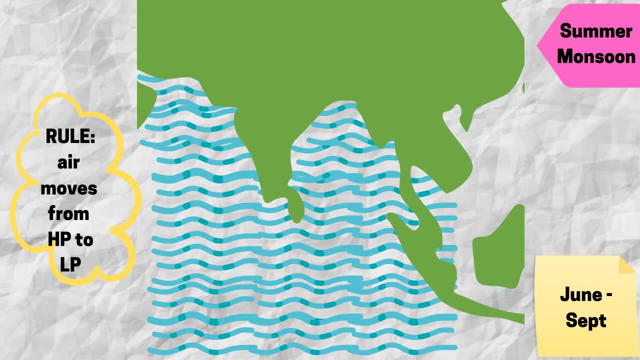 and drought. This is why our winter monsoon is also known as our dry monsoon. Let's compare this to the summer monsoon. In summer, the land gets a lot warmer. Warmer is associated with a low pressure cell, and so there is a low 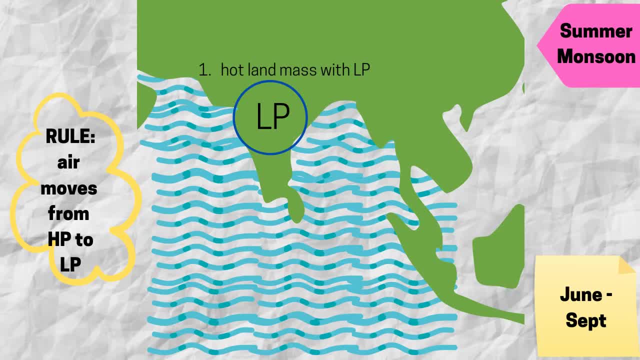 pressure over the land. In comparison, the ocean is much cooler. Colder air is associated with a high pressure cell. Remember our rule: Air always moves from a high pressure to a low pressure. That means that during a summer monsoon, air is moving from the ocean to the land. Have a. 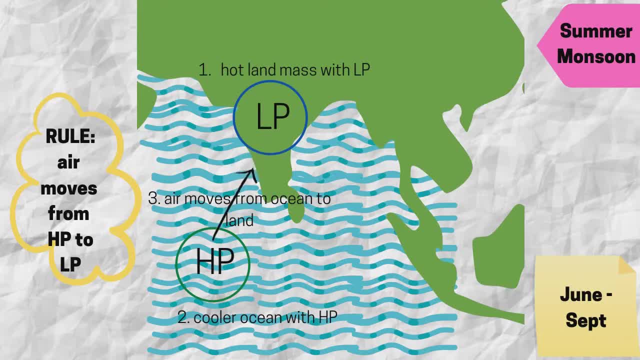 look where this wind is coming from. It is coming from the southwest. This is why the summer monsoon is also known as the southwest monsoon. When air comes from the ocean, it contains a lot of moisture. This air rises, cools and condenses.